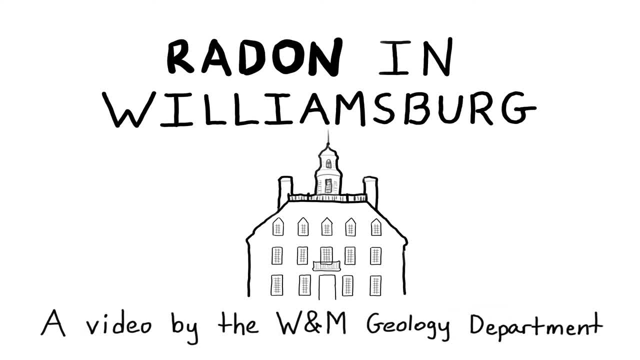 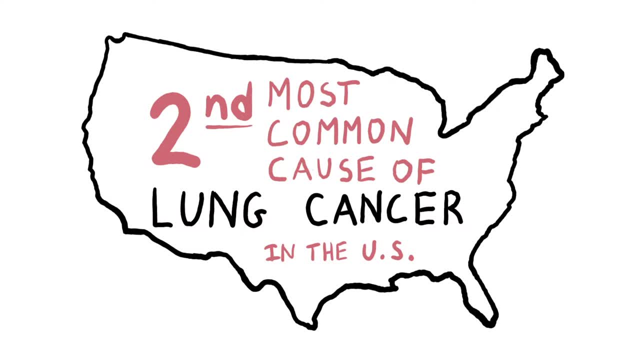 Did you know several homes in the Williamsburg area were found to have hazardous levels of radon and that radon is the second most common cause of lung cancer in the United States? This odorless, invisible gas does not cause immediate side effects, so you may or may not. 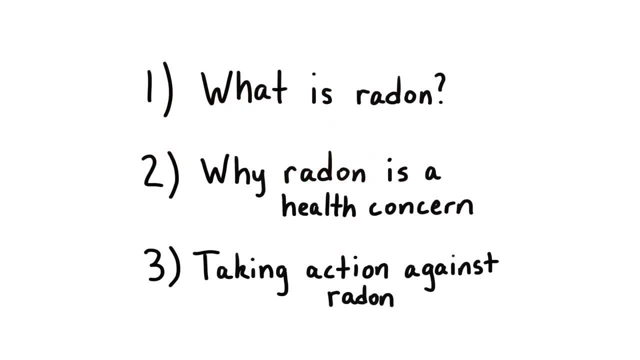 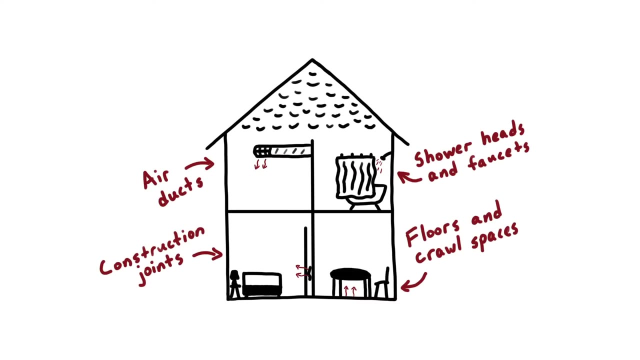 know if your household has been exposed. In this video, you'll learn what radon is, why it's a health concern and how you can take action to mitigate radon in your home. Radon is a naturally occurring radioactive gas that can enter your home from the ground through multiple points. 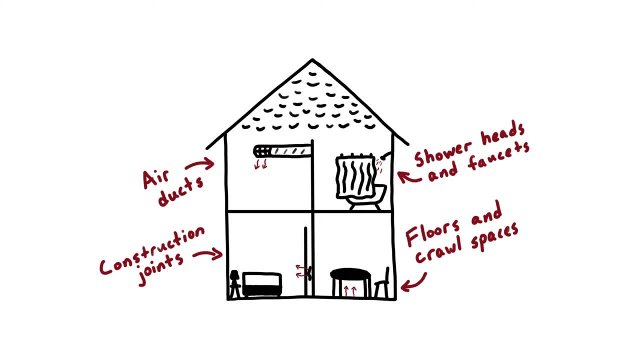 including air ducts, cracks in your walls, floors or foundation, crawl spaces, construction joints or your local water supply. The highest levels of radon are usually found in the lowest areas of a home. Radon levels can fluctuate with the seasons, with the highest levels usually. 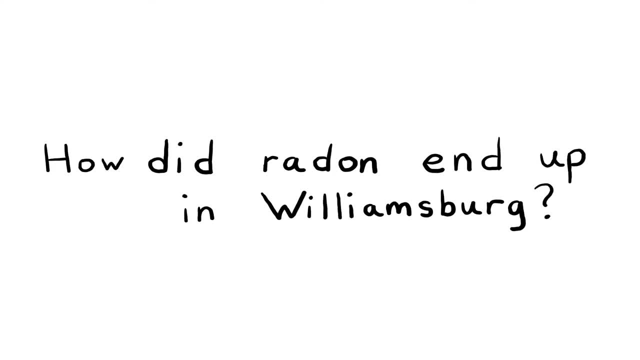 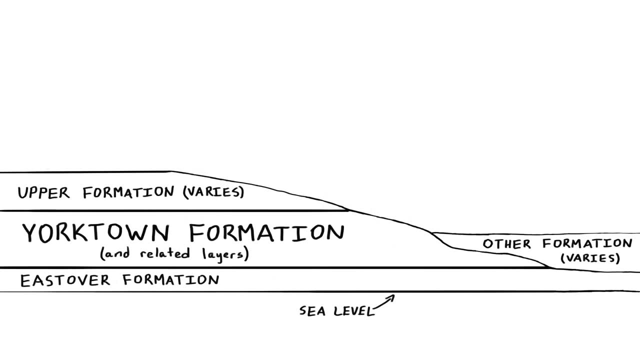 occurring during the winter months. But how did radon end up in Williamsburg? This explanation requires a little bit of research. If you're interested in learning more about radon, a brief geology lesson. The ground beneath our feet consists of multiple layers of sediment. 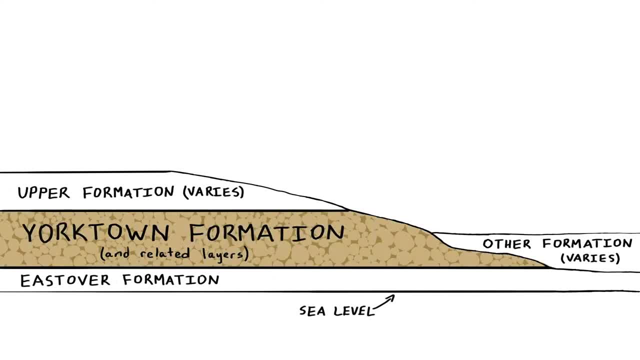 One of these layers, called the Yorktown Formation, is primarily composed of porous sand shells and marine mammal bones. It turns out that the fossils common in this formation, such as whale bones and shark teeth, are a key source of uranium. Uranium naturally decays into 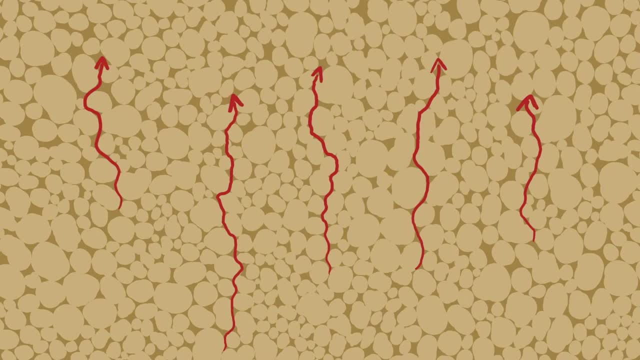 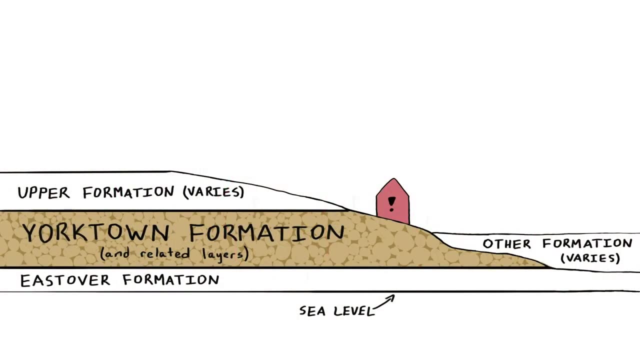 radon and, as a gas, can then escape between the grains of sediment and travel up to the surface. If your home is built on or near the Yorktown Formation, there could be radon seeping into your home without you even knowing it, And if you do have a radon problem. 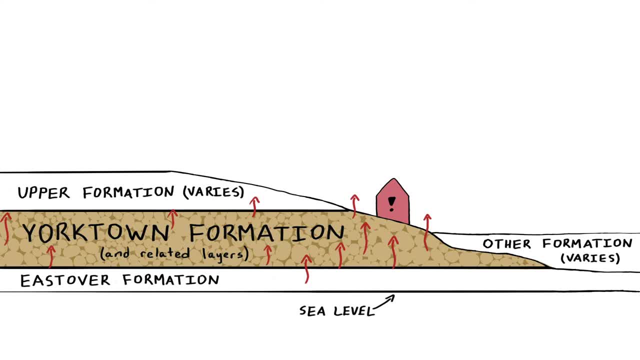 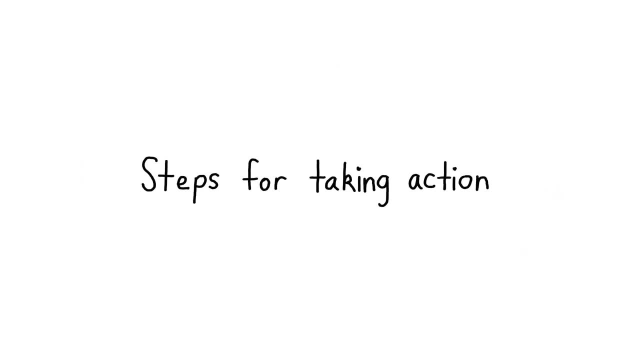 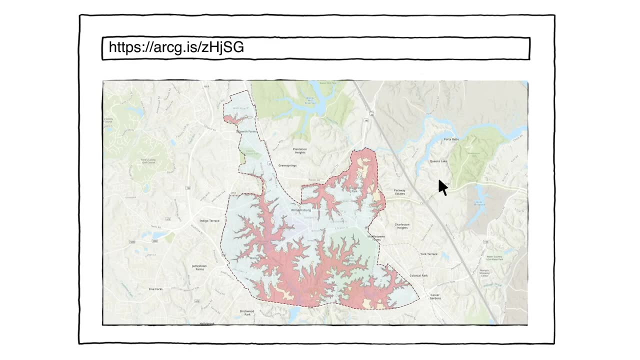 it's essential that you take immediate action to protect yourself and your loved ones. Rest assured, there are easy, affordable and effective solutions, and you can start right now. Simply follow these four steps. The William & Mary Geology Department has an online interactive radon risk map of Williamsburg. 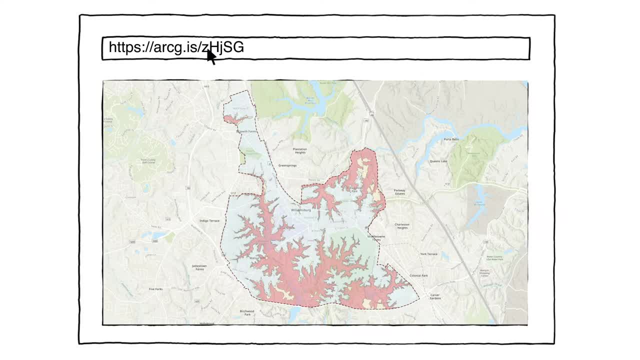 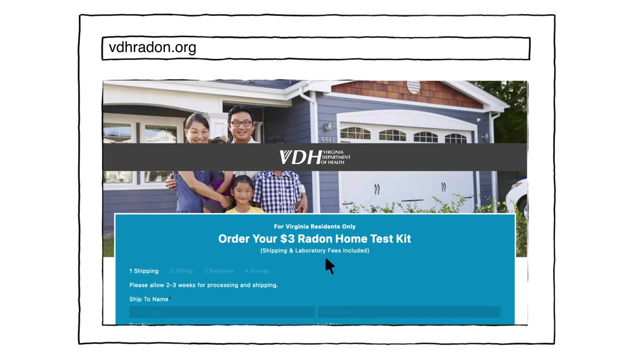 Follow the map link in the description to quickly determine your home's estimated level of risk. Obtain a radon test kit as soon as possible, especially if your home is in a moderate to high risk area. Testing is easy: The 2-3 day test only takes a few minutes to perform.